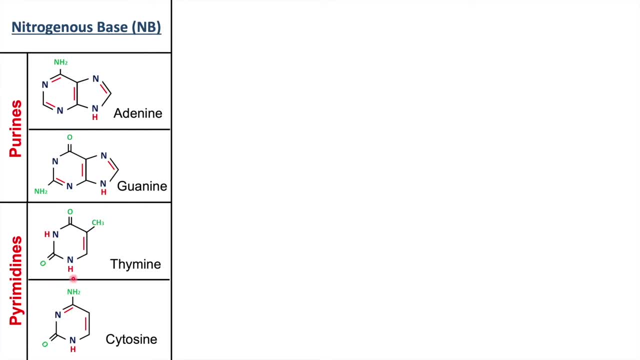 The second type of nitrogenous base is pyrimidine, and pyrimidine is a single ring because it's a six member carbon ring, And pyrimidines contain thymine and cytosine. So now when the sugar molecule is attached to this nitrogenous basis, it is called nucleoside. So basically, nucleoside is just the adding one sugar molecule into the nitrogenous base and then that becomes the nucleoside. 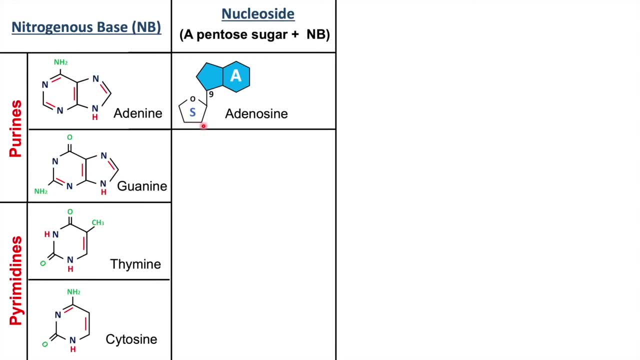 In case of adenine, when the sugar molecule is added to adenine, it becomes adenosine. And similarly, when the sugar molecule is added to the guanine, it becomes guanosine. And similarly for thymine: it becomes thymidine. And when the sugar molecule is added to cytosine, it becomes cytidine. 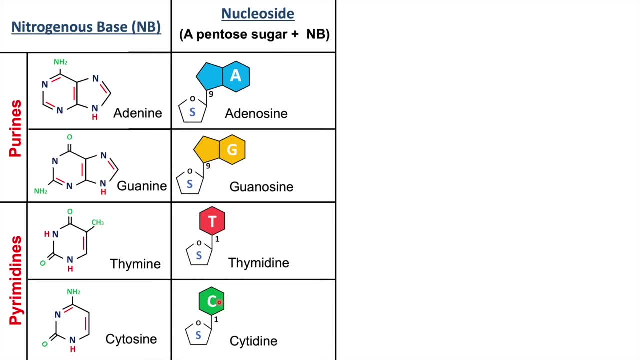 Now, lastly, when the phosphate group is added to a nucleoside, it becomes nucleotide. So, like we saw in the previous slide, nucleosides contain a phosphate group and a sugar and a nitrogenous base. So when the phosphate group is added to a nucleoside, it becomes nucleotide. 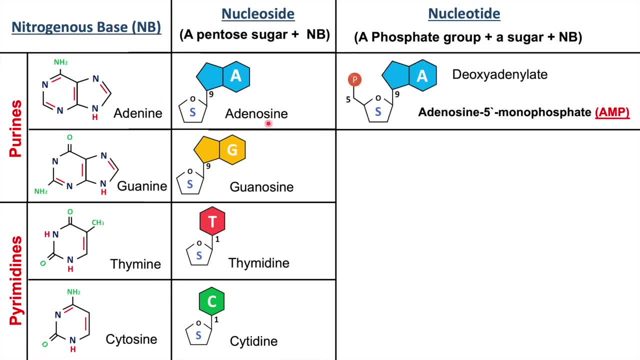 So let's see here: when the phosphate group is added to a nucleoside that is adenosine, it becomes deoxyadenolate. Now it is called deoxyadenolate in case of DNA, but if it's RNA, it will be called as adenolate. 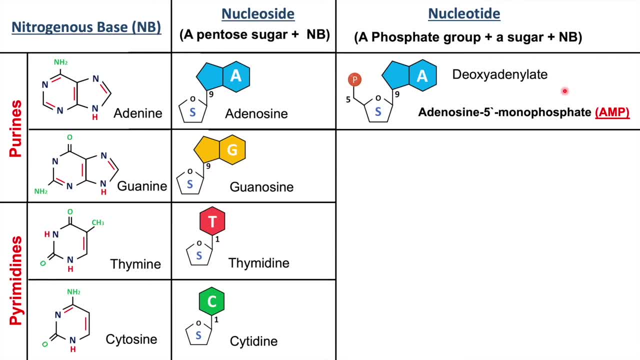 Now, here we are only going to focus on DNA, So that's why I'll be only referring to in terms of DNA. So, in addition to deoxyadenolate, it is, alternatively, it is also called as adenosine 5-monophosphate. Why? Because phosphate group is attached to the carbon 5 of the pentose sugar. That's why it is called adenosine 5 and monophosphate, because it is that there is only one phosphate group attached. That's why it is called monophosphate. 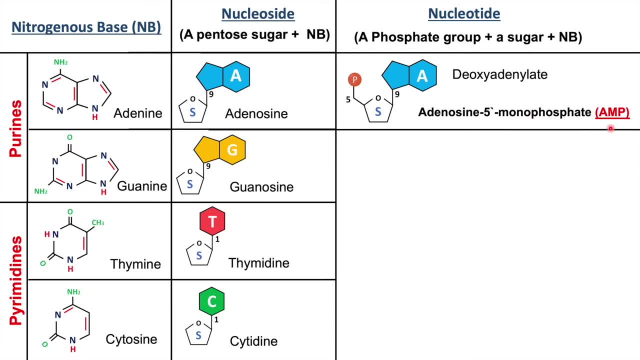 So adenosine 5-monophosphate, that is, AMP. Now when the phosphate group is attached to gonosine, it becomes deoxyagonalate And alternatively it is also called as gonosine 5-monophosphate, GMP. 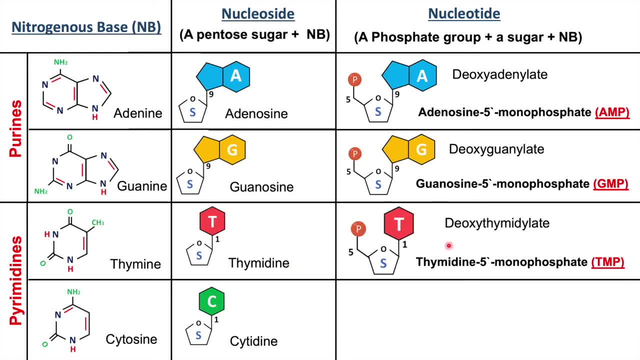 Now, when the phosphate group is attached to thymidine, it becomes deoxythymidylate or thymidine 5-monophosphate. that is TMP. And when the phosphate group is attached to cytidine, it becomes deoxycytidylate, or it is also called as cytidine 5-monophosphate. that is CMP. 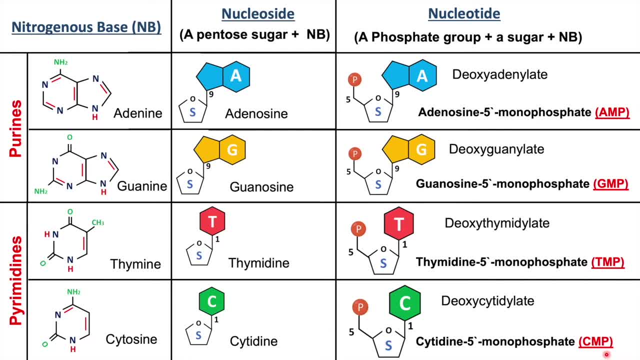 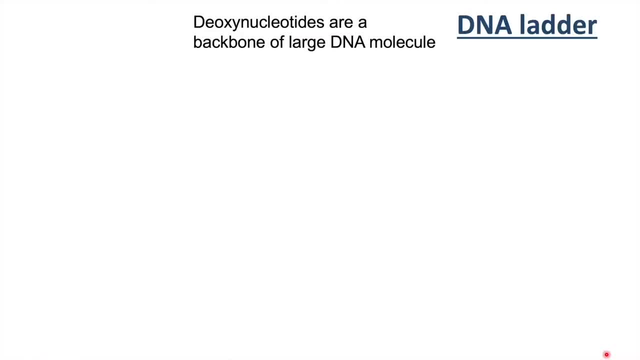 So if you want to review more on nucleic acids, nucleosides and nucleotides, please refer to my previous video. So so, these deoxynucleotides, or DNA nucleotides, are actually a backbone of larger DNA molecules. 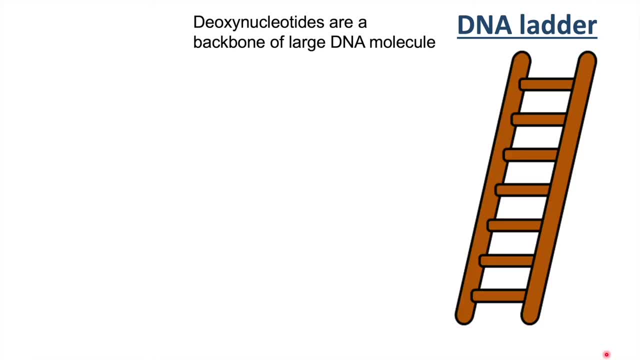 And when they are joined together they kind of resemble like a ladder And then therefore it is called a DNA ladder. So we are now going to build this DNA ladder, And to build this DNA ladder we are going to require nucleotides. 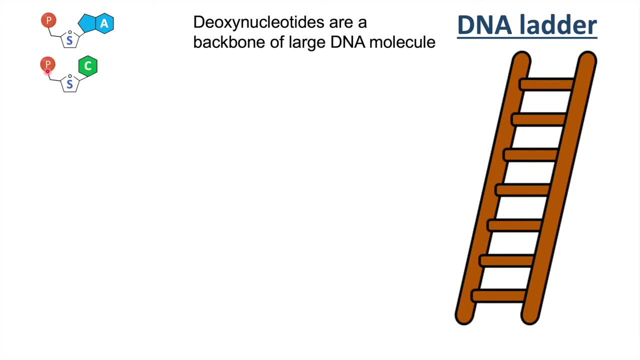 So here we have adenine, And we have cytosine And thymine, And now we need to connect these nucleotides, So the sugar of one nucleotide is connected to the phosphate group of the next nucleotide. So there is a bond formation between a sugar of one molecule, one nucleotide, and the phosphate group of the next nucleotide. 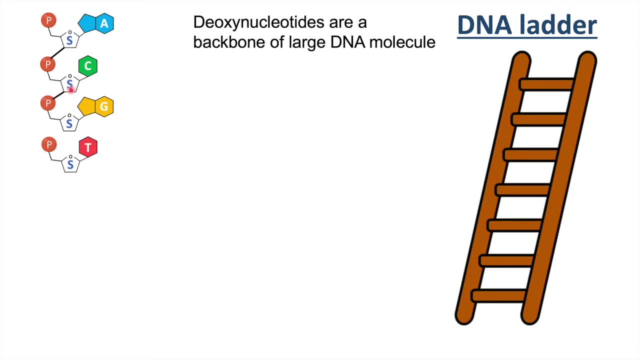 So, similarly, the cytosine is the sugar of the cytosine is connected to the phosphate group of the next nucleotide. So let's connect all these nucleotides and complete the one strand of DNA. So this is the one strand of DNA. 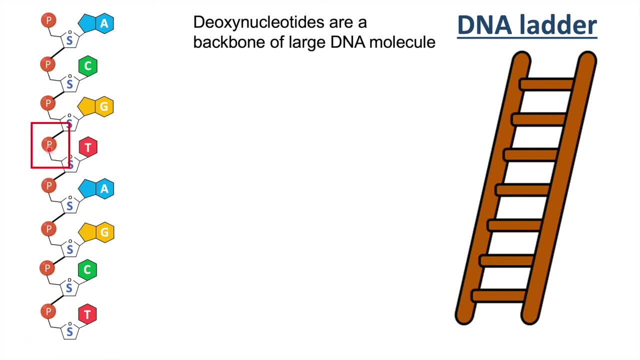 Now, if you notice here that this phosphate group is attached to a sugar molecule of one nucleotide- In this case it's a gonine- And it is also attached to a sugar molecule of the next nucleotide- In this case it's a thymine. 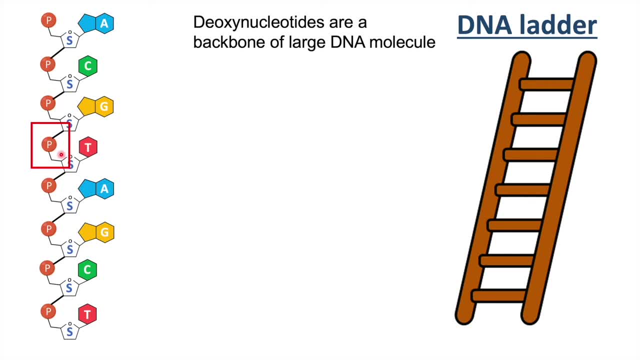 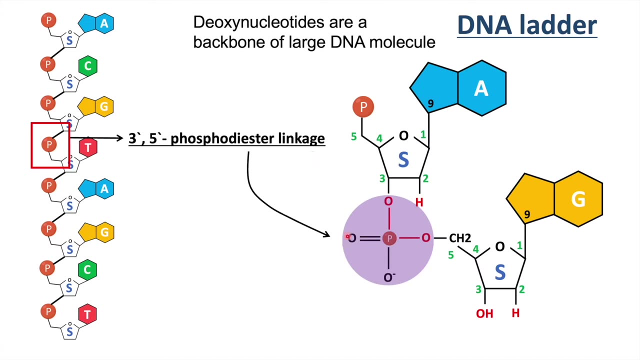 So this connection of phosphate bond, phosphate group- to the two sugar molecules is called 3,5-phosphodiester linkage. Why is it called 3,5-phosphodiester? Because the phosphate group is attached to three carbon of one sugar molecule from nucleotide adenine. 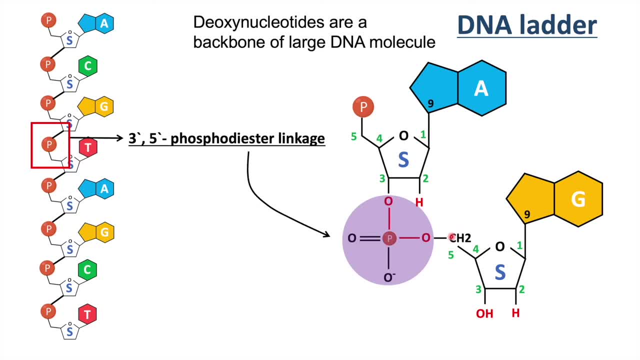 And it is also attached to, and the phosphate group is also attached to carbon 5 of the other sugar molecule from the nucleotide gonine. So that's why- because it is attached on one sugar molecule at carbon 3, and it is also and the phosphate group is also attached to another sugar molecule at carbon 5.. 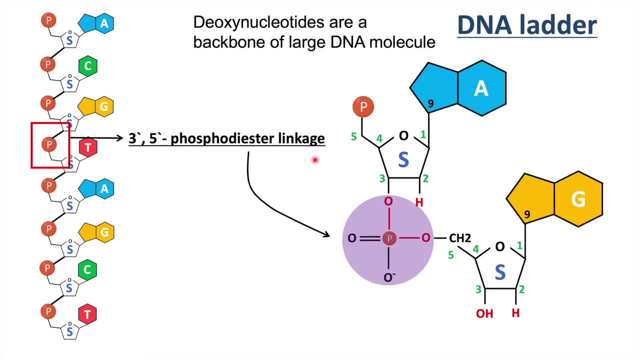 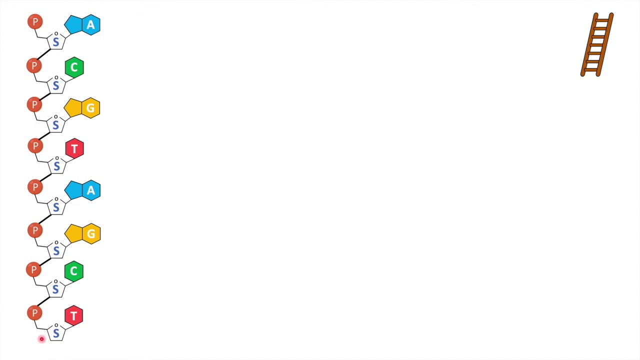 Therefore it is called 3,5-phosphodiester linkage, And it is in fact a covalent linkage, because the covalent bond is formed whenever two atoms are connected to each other by means of sharing electrons. So now here we have one DNA ladder. 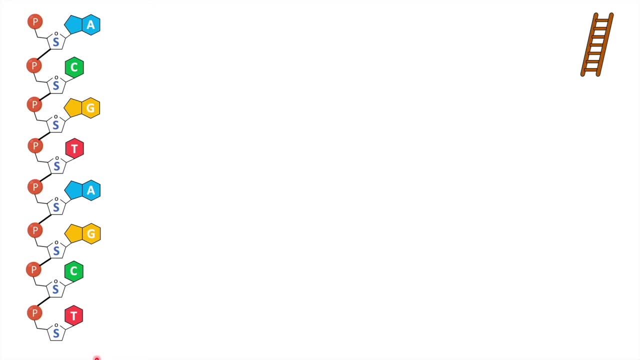 Now, DNA is a double stranded molecule, So we also need to now make the second DNA strand. So let's now draw the second DNA strand. So to draw the second DNA strand, we need to keep in mind that adenine is always pairs up with thymine and cytosine always pairs up with gonosine. 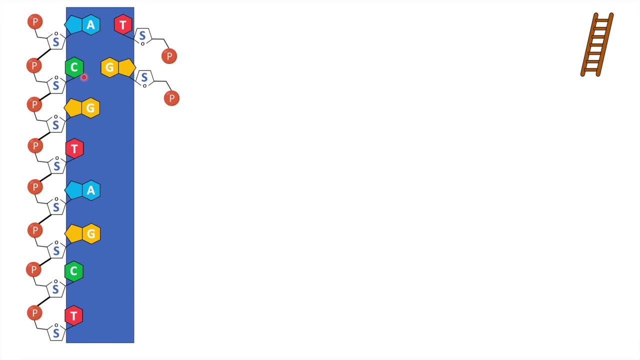 And this pairing of adenine to thymine and cytosine to gonine it's called complementary base pairs, meaning that adenine of purine must always pair with thymine of pyrimidine And also the cytosine of pyrimidine must always pair with gonine of purine. 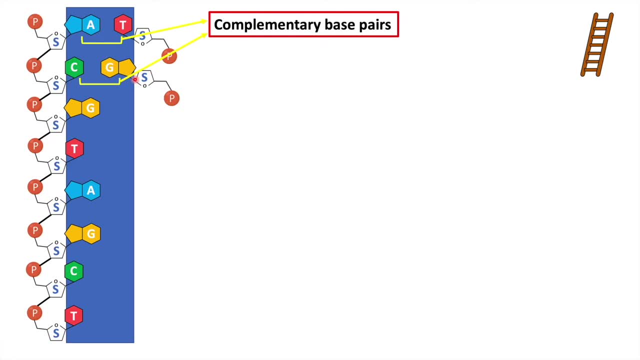 So it is important to remember that these are called complementary bases because adenine pairs up with thymine and cytosine pairs up with gonine. Now let's complete the remaining strand. So here, as per the complementary bases, we can now build up the second strand. 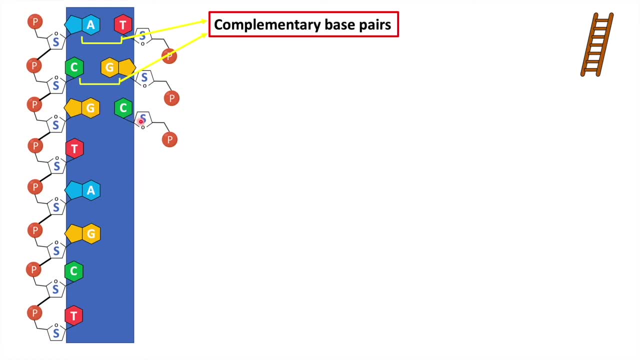 So opposite to gonine we have cytosine, Opposite to thymine we have adenine, And opposite to adenine we have thymine, then cytosine, then gonine, And again opposite to thymine we have adenine. 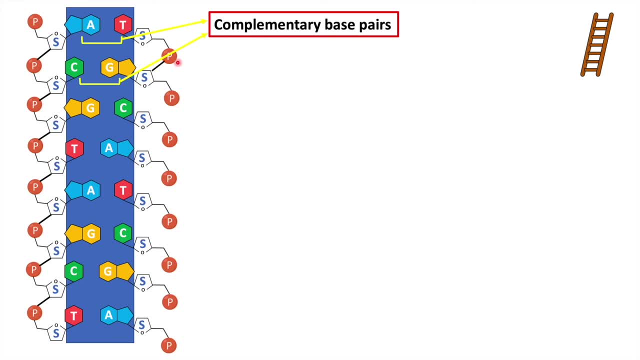 And again, these nucleotides are connected to each other via phosphodiester linkage, So we have also connected these nucleotides Now. the other thing to remember in these DNA strands is that on the left side of the DNA strand, you can see that the sugar molecule is facing up. 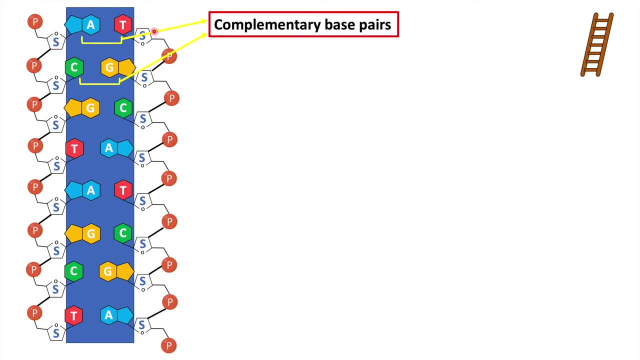 whereas on the right side of the DNA strand, the sugar molecule of the nucleotide is facing down. So this is also an important thing to remember. And the other thing to keep in mind is that if you know the nucleotide sequence of the left side of the DNA strand, 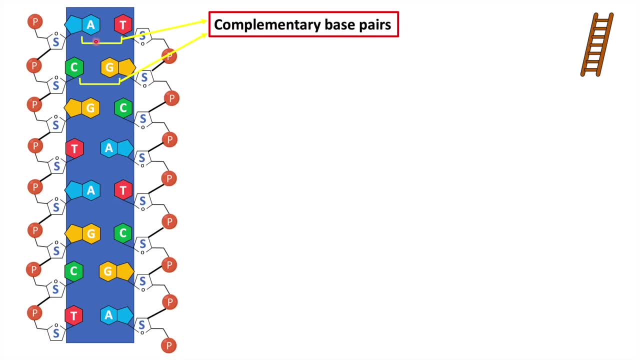 you should be able to draw the opposite side of the DNA strand And therefore this is called a complementary strand, Because if you consider the left side of the DNA strand as a starting material, you should be able to draw the complementary DNA strand on the opposite side. 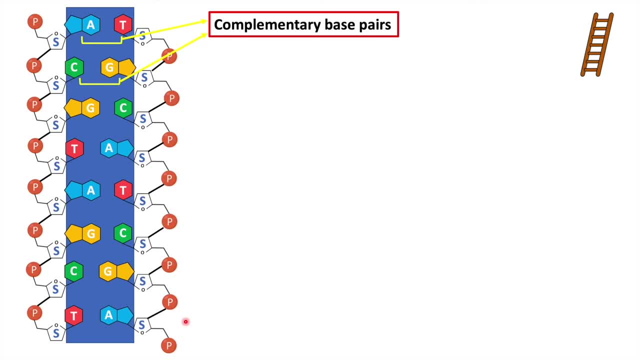 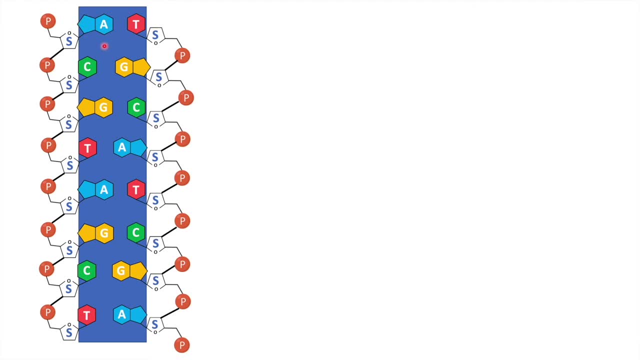 And therefore it is called a complementary DNA strand. So now the important thing is how these complementary base pairs are joined together, or how they are connected to each other. So if we focus on the first one, adenine and thymine- 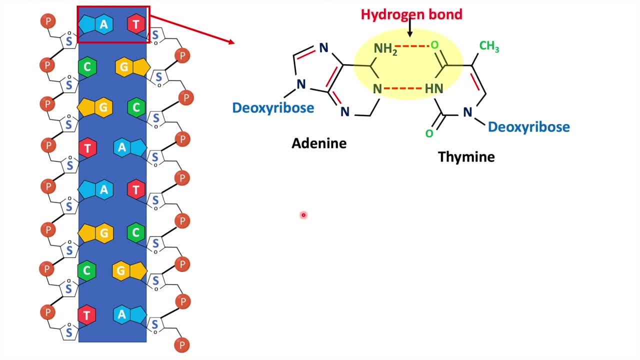 both adenine and thymine are connected to each other via a hydrogen bond And these hydrogen bonds are formed between the hydrogen atom of one base And. this hydrogen atom acts as a hydrogen bond donor And it is connected to the or it forms a bond with the. 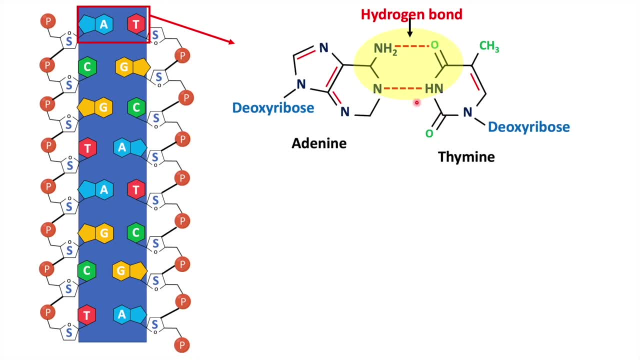 oxygen atom, either an oxygen atom or nitrogen atom of the opposite base, And here the oxygen atom and the nitrogen atoms are acts as a hydrogen bond acceptor. So these are non-covalent hydrogen bonds, and it is important to remember that there are two hydrogen bonds between adenine and thymine. 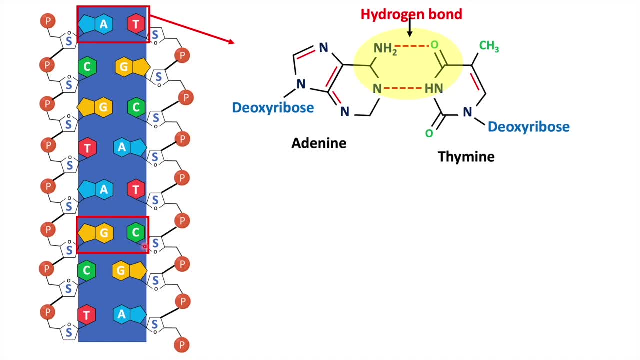 And likewise there are three hydrogen bonds between gonine and cytosine. So this is important to remember: that there are only two hydrogen bonds between adenine and thymine, whereas there are three hydrogen bonds between gonine and cytosine. 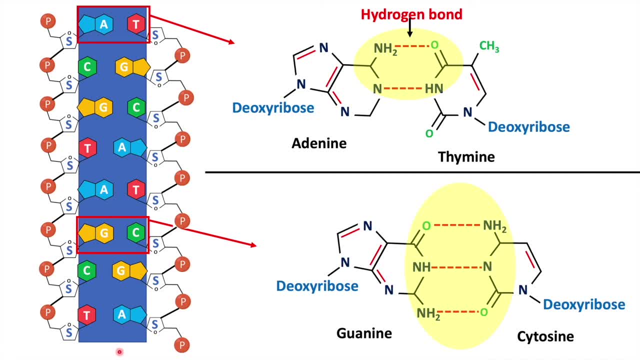 So now let's complete our DNA strand by forming the hydrogen bond between these nitrogenous bases. So, as we saw, there are two hydrogen bonds between adenine and thymine, three hydrogen bonds between gonine and cytosine, And this is the rest of the ladder. 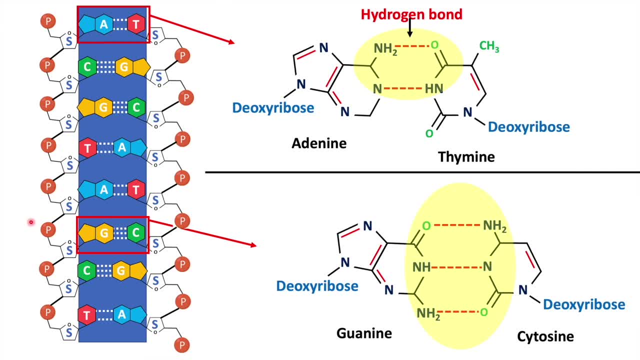 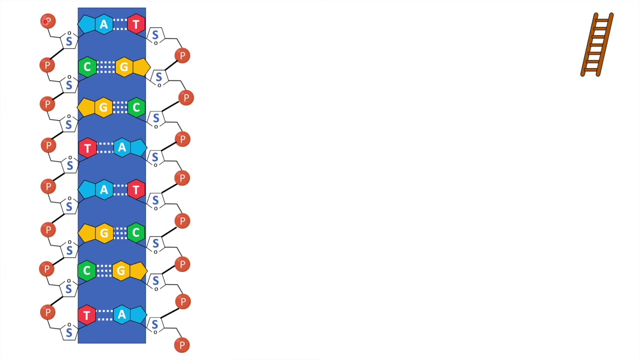 So now our DNA ladder is completed And it is these hydrogen bonds which actually connects the two strands of the DNA And, most importantly, these hydrogen bonds also provide the stability to the DNA molecule. So this is the complete DNA ladder, So the alternating phosphate group and sugar molecule. 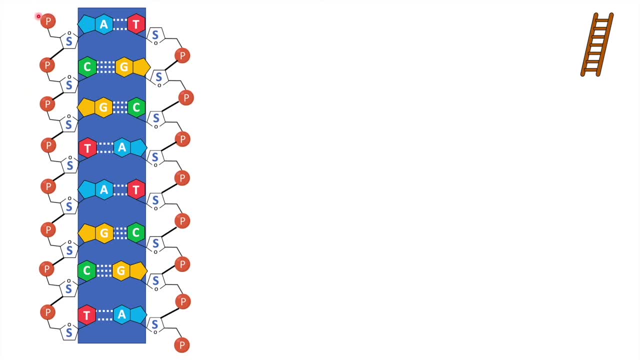 so these are the backbone of sides of the ladder. So phosphate and sugar the one strand And on the other side phosphate and sugar, that is the second strand. So these are kind of forms, the backbone of the sides of the ladder. 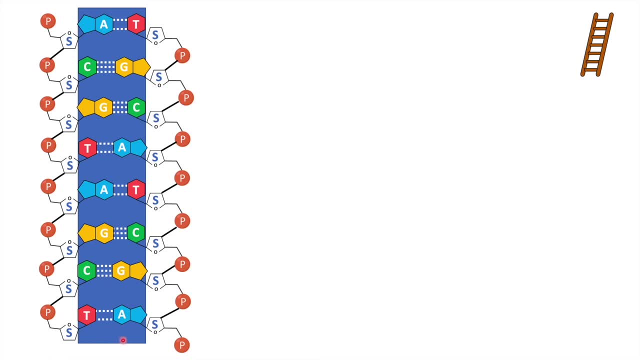 And the one in the blue where nitrogenous bases are attached to each other. those are the rungs, or the steps, which are the central part of the DNA ladder, And the sides of the DNA ladder are, as we have seen before, that they are made up of alternating phosphate group. 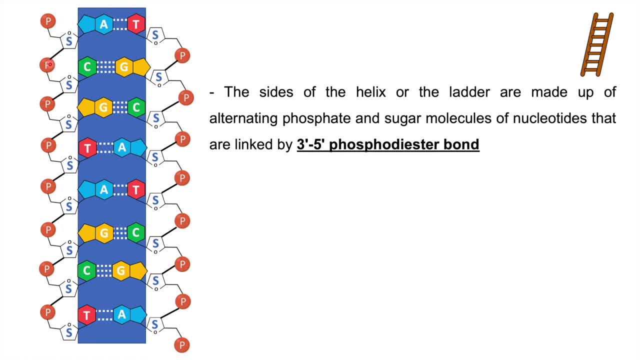 and the phosphate group of one nucleotide and a sugar molecule of the next nucleotide, And they are linked together via 3,5-phosphodiester bond, And the rungs or the steps of the DNA ladder are made up of paired complementary nitrogenous bases. 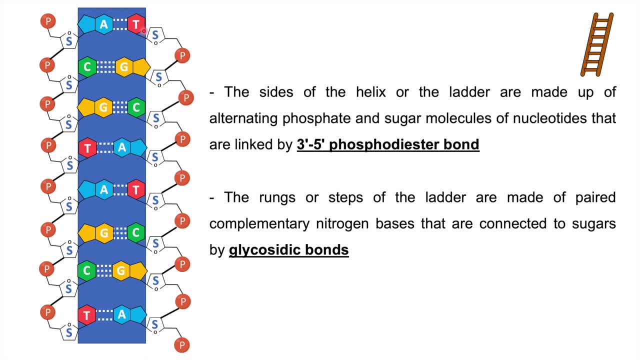 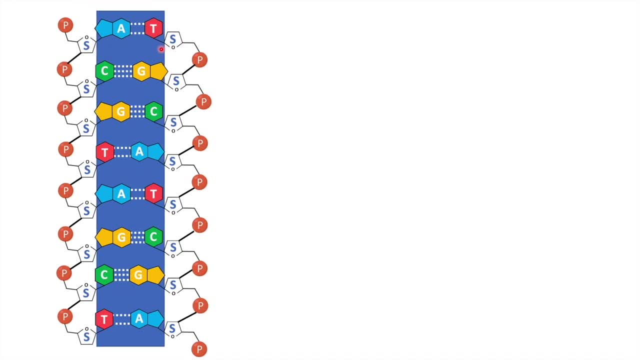 And it is also important to know that these nitrogenous bases are connected to a sugar molecule by glycosidic bonds. Now, next, we also need to know that, because of the complementary base pair, the number of adenines are equal to the number of thymine. 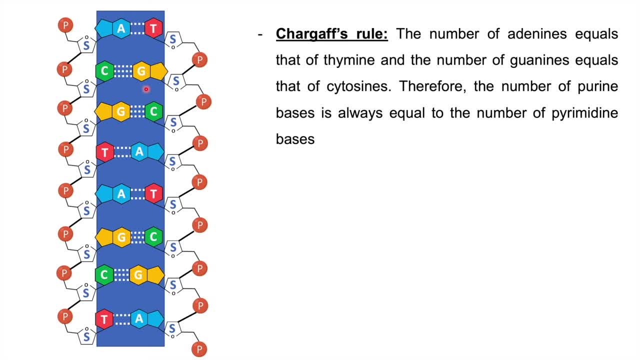 and also the number of cytosines are equal to the number of gonines because they are complementary bases. so it is the number of adenine and thymine are always going to be equal and the number of cytosine and gonine are always going to be equal. 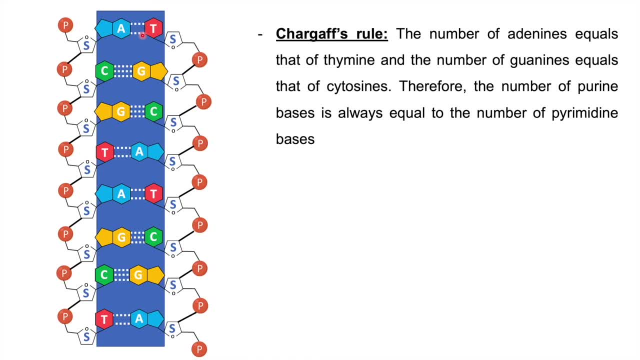 And because, and then therefore, the number of purine bases is also equal to the number of pyrimidine bases, because adenine is a purine ring, whereas thymine is a pyrimidine ring. So this is also that means the number of purines and pyrimidine bases are also equal. 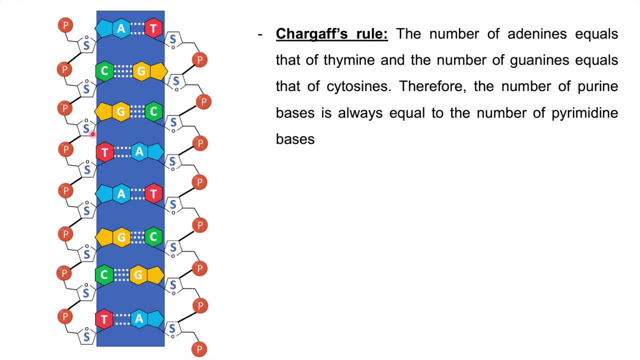 And and. secondly, these DNA strands can be separated by melting this strand at a certain temperature. However, the important thing to remember- that DNA which has a high GC content means which has a high gonine and cytosine nitrogenous bases, requires a higher melting temperature compared to the 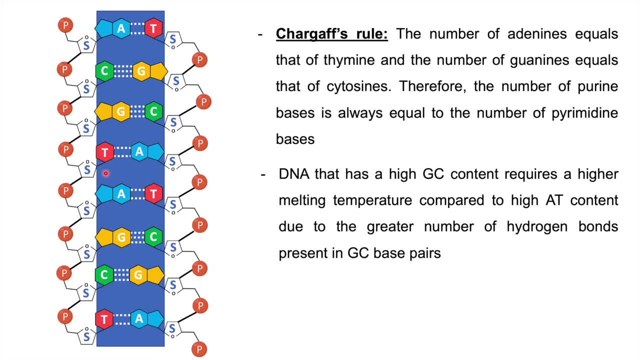 compared to the ANT content or compared to the content of thymine and adenine, because GNC, or the gonine and cytosine, have higher hydrogen bonds to break compared to the hydrogen bonds between adenine and thymine. So therefore GNC requires a higher melting temperature compared to the 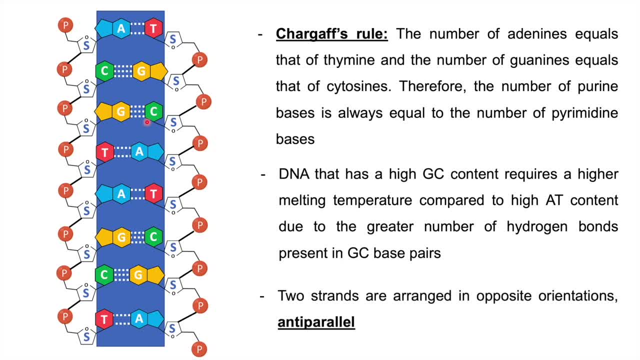 ANT. Now, the last thing is also important: that these two strands are arranged in opposite orientation and that's why they are called anti-parallel. Why? Because if you, if you pay attention on the left side of the strand, left side of the strand starts with the phosphate group. 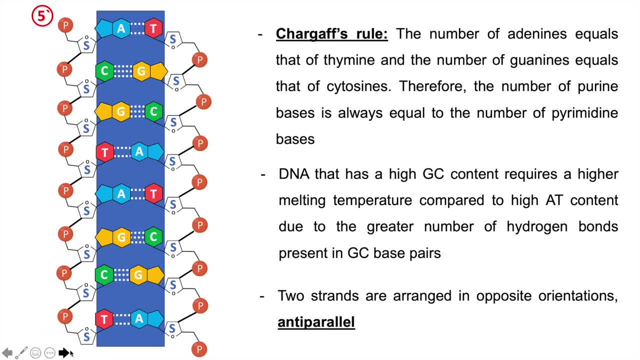 which is attached to the 5 carbon of the sugar molecule, whereas it ends with the 3 carbon of the sugar molecule. So, therefore, it runs from 5 prime to 3 prime direction on one side, Whereas on the opposite strand it starts with the 3 carbon of the sugar molecule, whereas it ends with the 5 carbon. 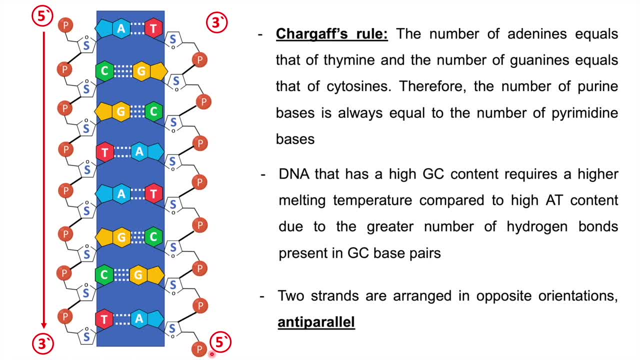 where the phosphate molecule, phosphate group, is attached, And therefore it also runs from 5 prime to 3 prime direction, but it runs in the opposite direction compared to the first strand. So therefore these strands are called anti-parallel strands. So now here we have two strands of DNA which looks very similar to a ladder. 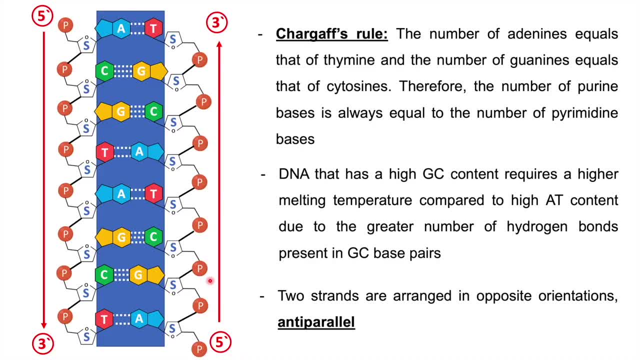 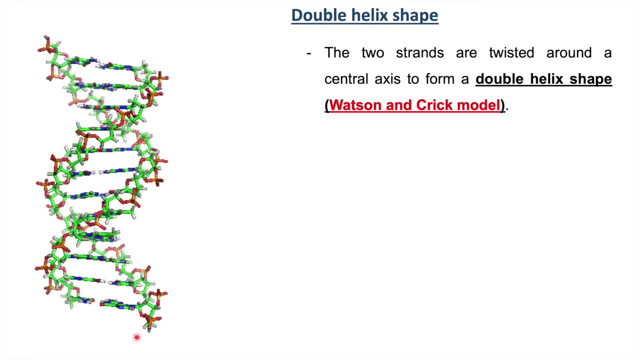 So, however, this is not the actual shape of DNA. In fact, the two strands of DNA are twisted around to a central axis to form a double helix shape of DNA. So this is the double helix shape of DNA, where the two strands are twisted around. 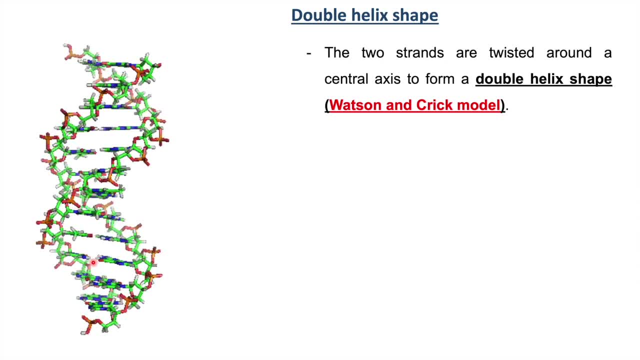 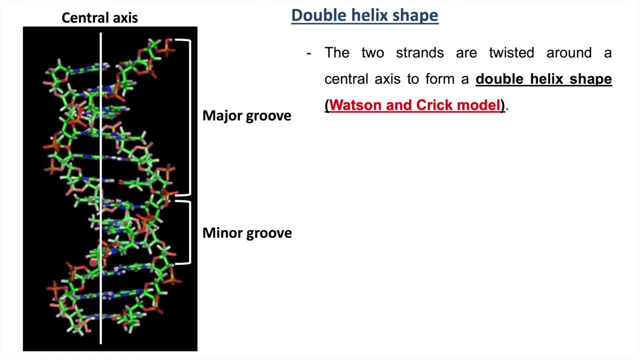 And this is a model which was proposed by Watson and Crick. That's why it is called a Watson and Crick model. So when they twist around each other, these two strands, when they twist around they form a major groove and a minor groove. 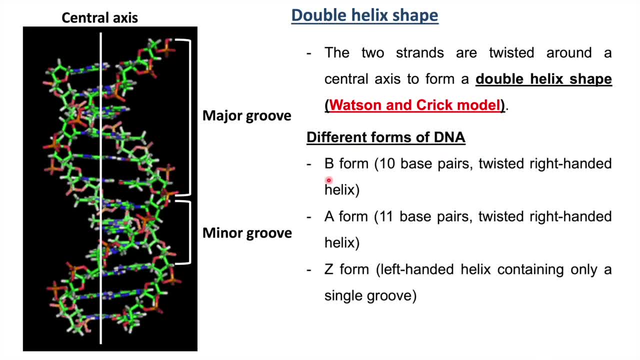 Now there are basically different forms of DNA. First is B form, which is actually proposed by Watson and Crick, and this is very common in humans. So this B form DNA has 10 base pairs, So when the one twist of this ladder consists of 10 base pairs, 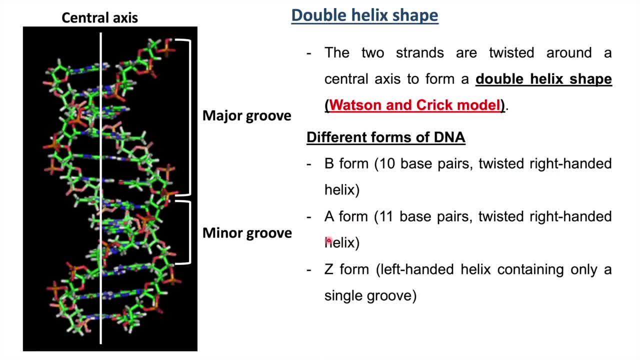 and it's twisted in the right-handed helix. Now there is another form, which is called A form. Now this form is more condensed because it contains more base pair, that is, 11 base pair, and this is also twisted right-handed helix, And the very rare form which is a Z form, where the